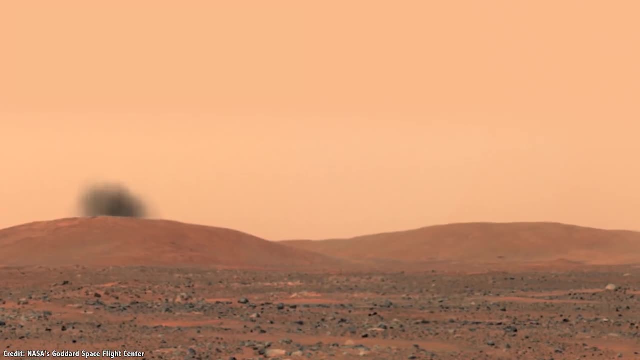 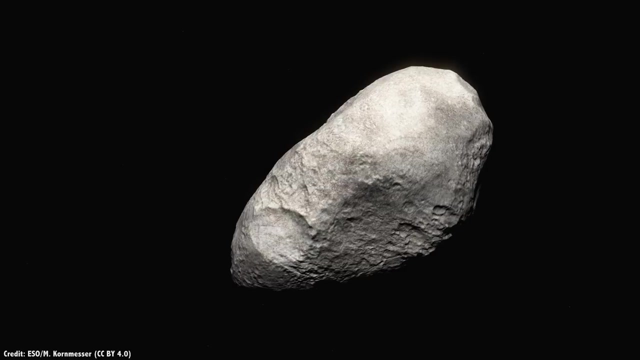 off into space faster than Mars' escape velocity. Some of this material orbited into the inner solar system and ALH4001 entered the Earth's atmosphere about 11,000 years ago, getting scooped up in 1984 by meteorite hunters. 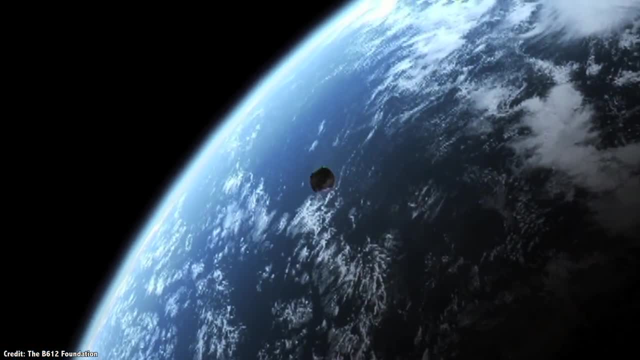 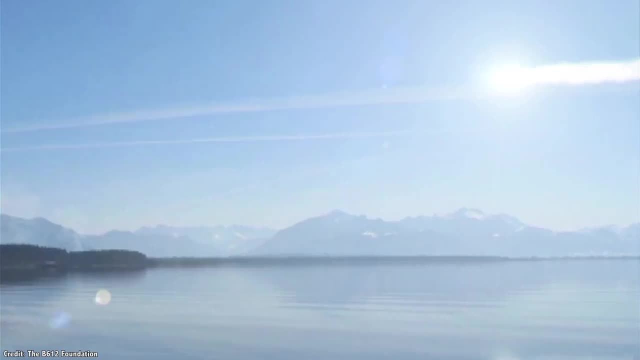 In fact, this has happened a lot. There are more than 70 Martian meteorites in the hands of scientists. In fact, this has happened a lot. There are more than 70 Martian meteorites in the hands of scientists. One surprising discovery is how well various lifeforms can withstand the extreme conditions. 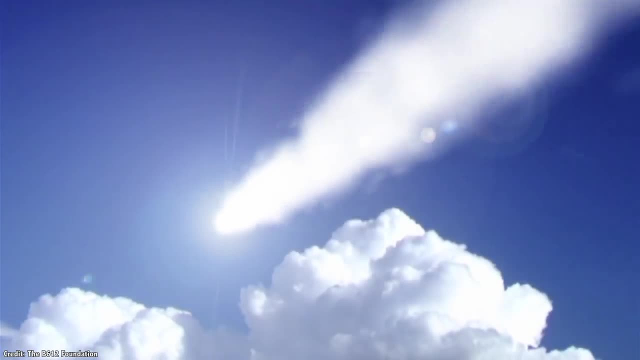 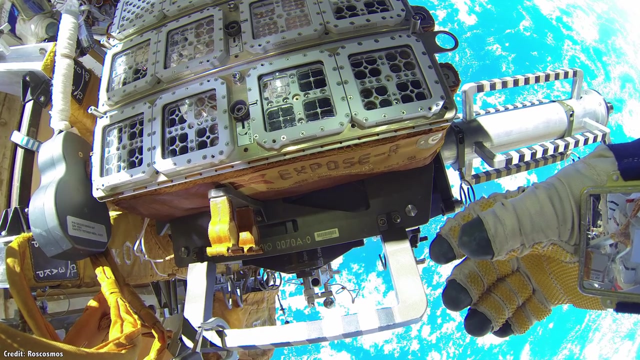 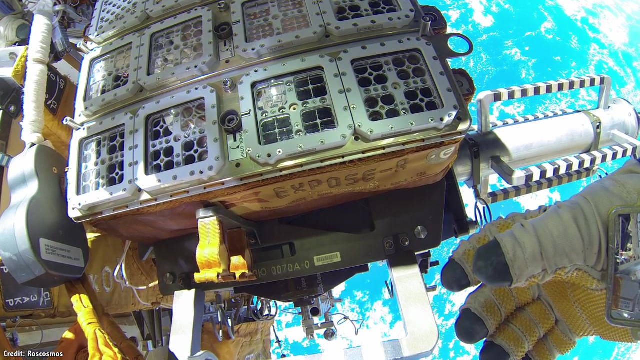 of space and then spring back to life when they return to Earth-like or even Mars-like conditions. In an experiment from 2014 to 2016, samples of various Earth lifeforms, from fungi to cyanobacteria, were exposed to the vacuum, extreme temperatures and ultraviolet radiation. 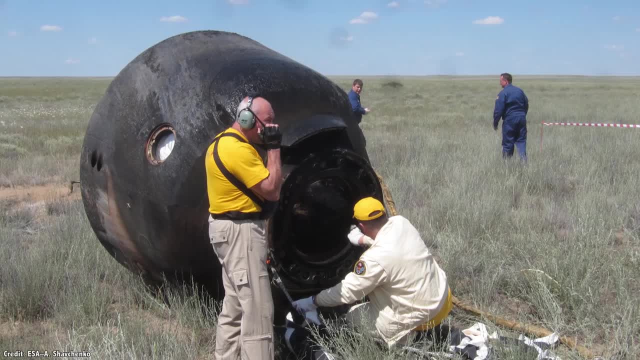 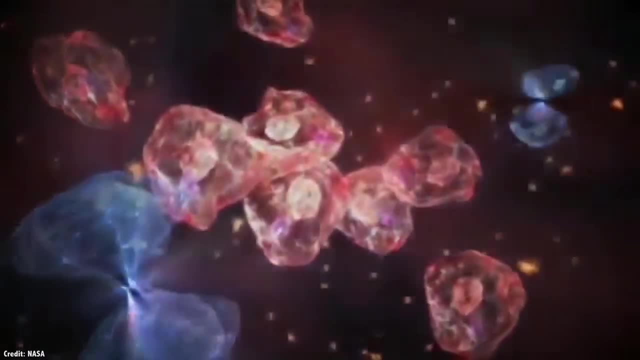 After they were brought back to Earth. they were brought back to Earth. they were exposed to the vacuum, extreme temperatures and ultraviolet radiation of space itself. outside the International Space Station experiment. it could still be a source of complex organic molecules and give life a 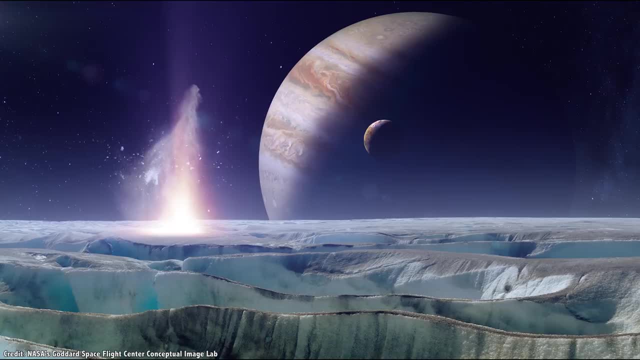 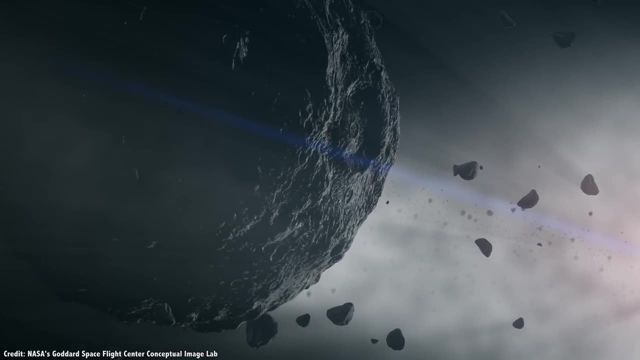 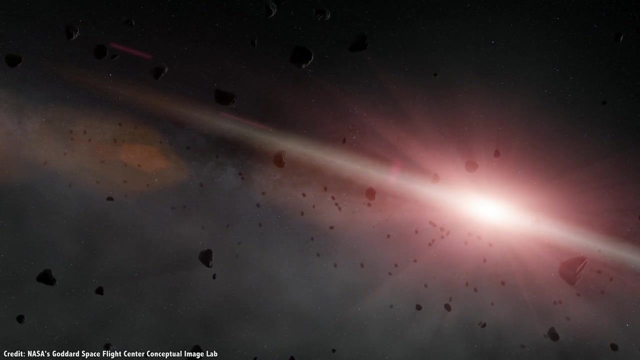 kickstart in another world. The term for this idea is necropanspermia. In theory, life could be protected inside rocky objects as small as one meter across, But these would be too difficult to push with light pressure alone. You need objects smaller than a millimeter to escape the pull of the sun. 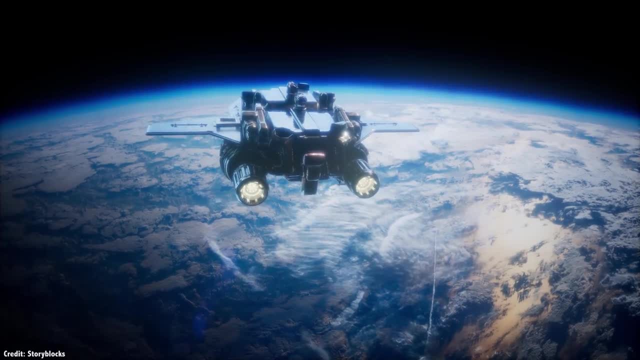 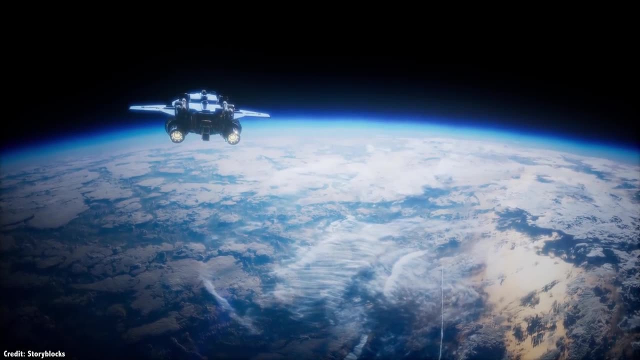 Of course. one last idea is that life is being intentionally seeded from world to world by aliens. This is known as directed panspermia. But come on, once you say aliens did it, the argument is pretty much over. Aliens could have done anything. 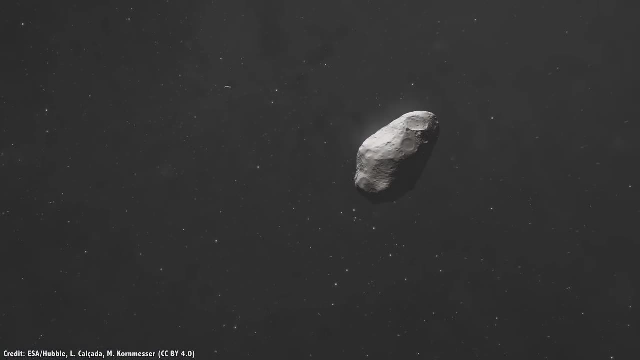 Or nothing. We've talked about how difficult it would be for meteorite impacts to send debris out into the galaxy, But there might be another way Comets- And we'll talk about that in a second, But first I'd like to thank Sebastian Hafenberg, Daniel Lieferink and the rest of our 842. 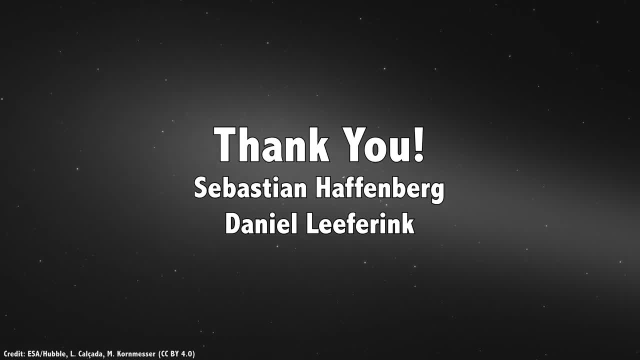 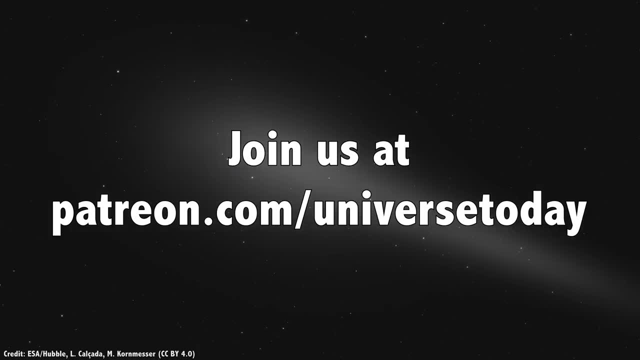 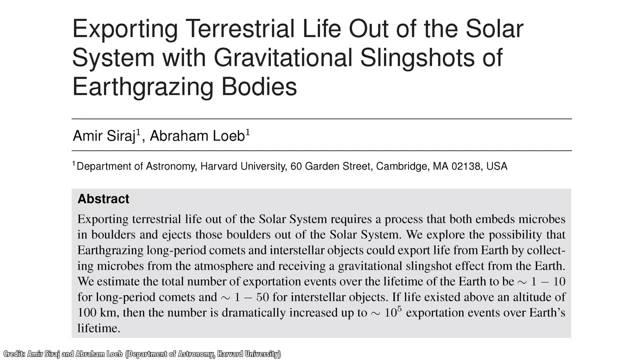 patrons for their generous support. Educational content You can be freely available to anyone in the world, and the patrons make this possible. Join our community at patreoncom slash universetoday and get in on the action. Amir Siraj and Avi Loeb recently wrote a paper called Exporting Terrestrial Life Out of the 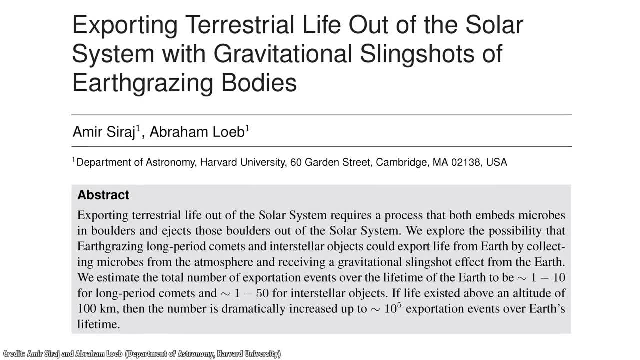 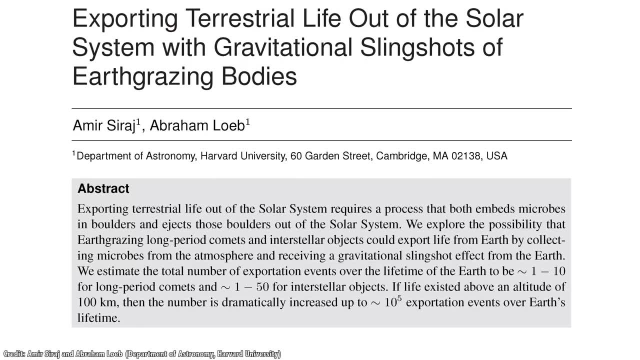 Solar System with Gravitational Slingshots of Earth-Grazing Bodies, And well, I guess the title really explains it all. there They looked into whether it could be possible for asteroids or comets skimming through the Earth's atmosphere to carry biological material out into the galaxy. 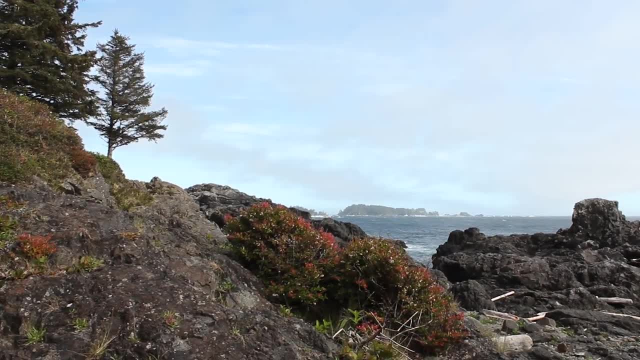 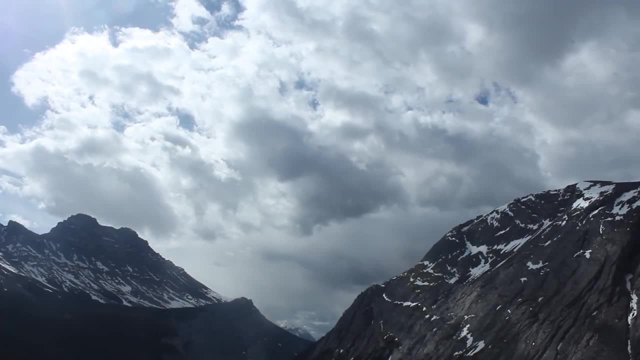 Life on Earth is mostly on the ground and in the oceans, but some of it is also in the atmosphere. In fact, microorganisms have been discovered at altitudes as high as 77 kilometers. This is high enough that a long-period comet from the Oort cloud could just graze the Earth's. 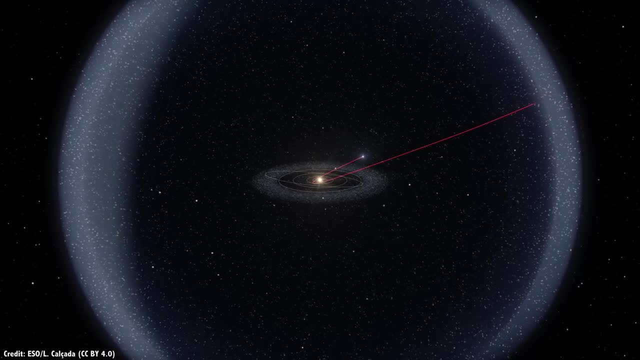 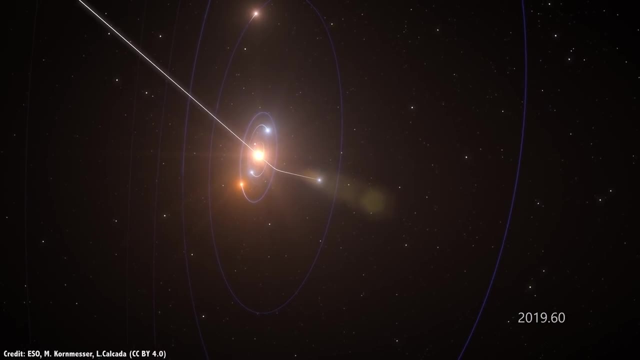 atmosphere, scoop up a face full of bacteria and then fly out into deep space again. And if that comet encounters a planet or large object in the Kuiper belt, it could be kicked out into an interplanetary trajectory that takes it from the sun to the moon. And if that comet encounters a planet or large object in the Kuiper belt, it could be kicked out into an interplanetary trajectory that takes it from the sun to the moon. And if that comet encounters a planet or large object in the Kuiper belt, it could. be kicked out into an interplanetary trajectory that takes it from the sun to the moon. And if that comet encounters a planet or large object in the Kuiper belt, it could be kicked out into an interplanetary trajectory that takes it from the sun to the moon. 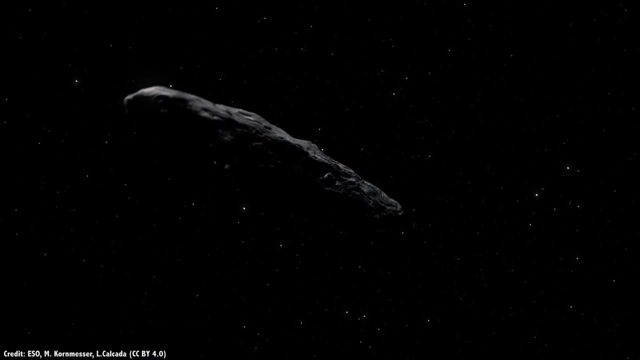 Thanks to Oumuamua and Comet 2i Borisov, we know that comets can get kicked out of their star systems and make an interstellar journey. In fact, there could be thousands of objects in the solar system right now. Siraj and Loeb simulated what might happen if a long-period comet passes through the. 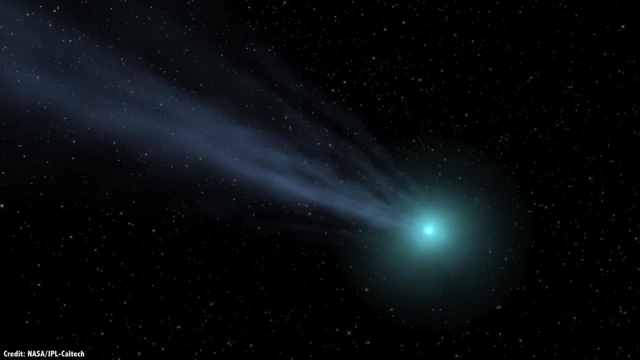 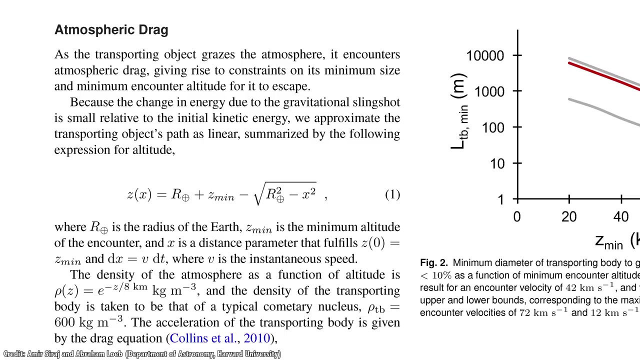 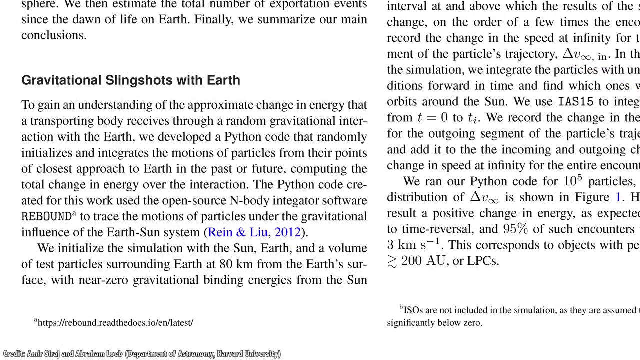 Earth's atmosphere. These objects are key because they just barely hold in orbit around the sun and it doesn't take much to kick them into an interstellar trajectory. They calculated how much atmospheric drag the objects would receive as they passed through the atmosphere, and also how much of a gravity slingshot they'd get. 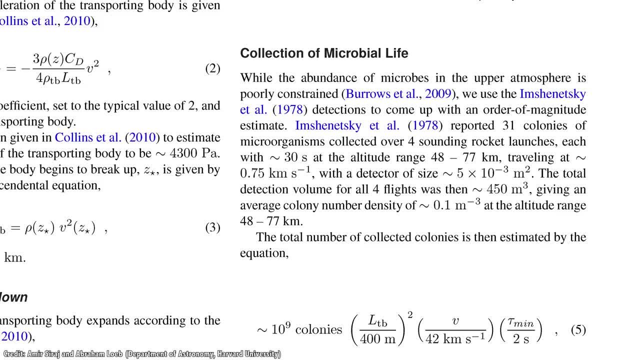 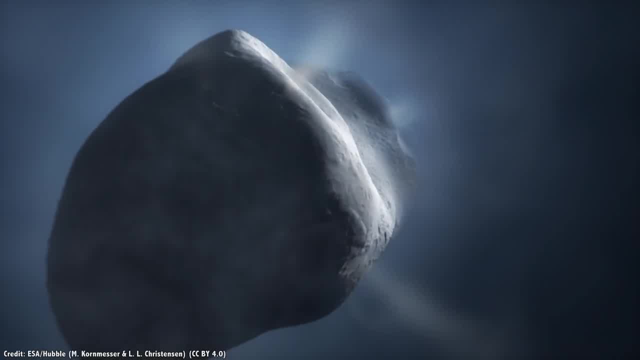 And they also determined how many bacteria would get scooped up by a comet as it passed through the atmosphere. Incredibly, bacteria can easily handle the kinds of instantaneous acceleration you'd get. slamming into a comet, screaming through the atmosphere hundreds of thousands or even 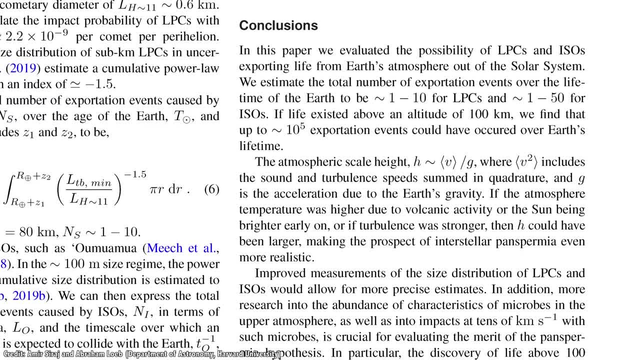 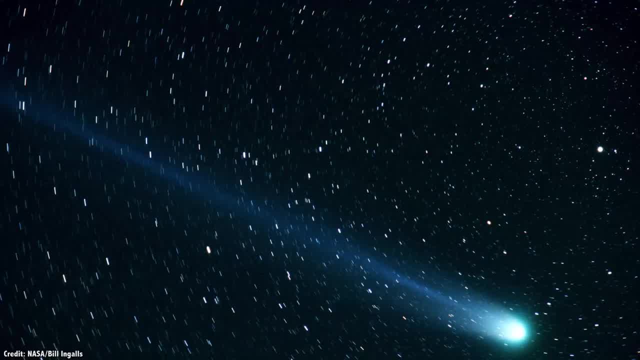 millions of Gs of force, And, based on their calculations, they estimated that this event could have happened up to 100,000 times in the history of the Earth. Now, we haven't had a bright comet visible in the northern hemisphere's night sky since. Hakutake back in 1996, and that was 15 million kilometers away. Imagine seeing a comet pass right through the Earth's atmosphere. Live long enough and you might see that happen. It's got to wait 45,000 years or so. 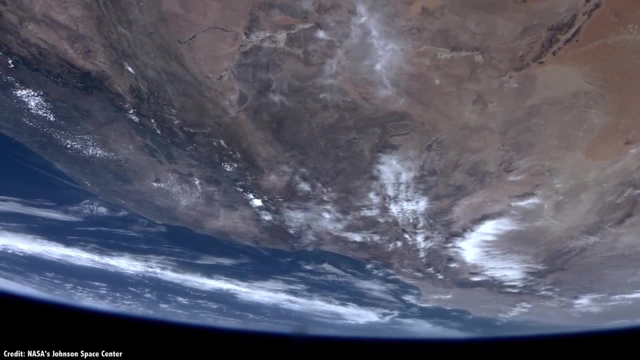 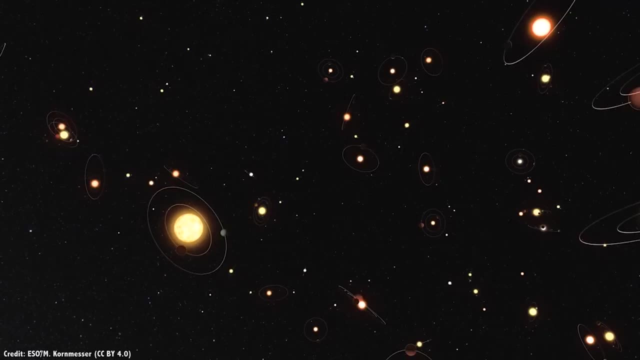 And if life is ever found Floating as high as 100 kilometers in the Earth's atmosphere, Siraj and Loeb think that it would dramatically increase the number of escapees. Think of the trillions of planets across the Milky Way and the comets carrying living material. 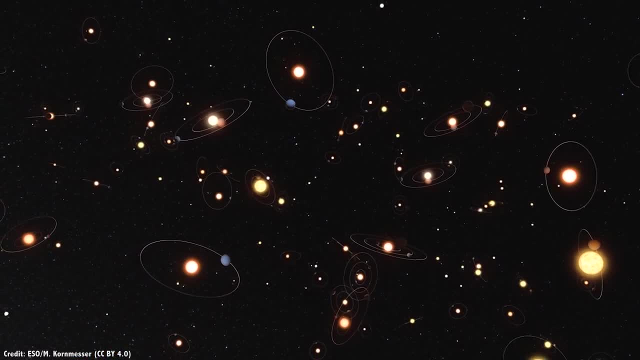 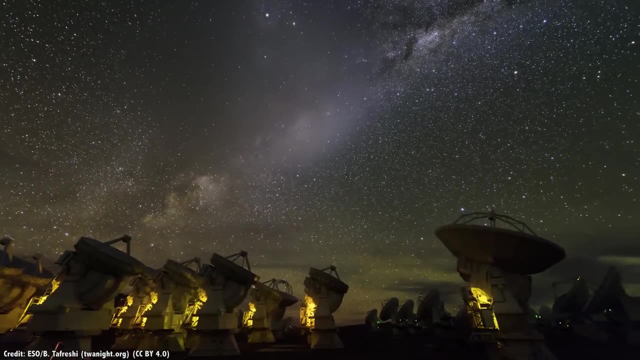 on an escape velocity out of all those star systems, and it makes you wonder if all life in the galaxy might be related. Of course, if there is life across the Milky Way, we don't see any evidence of advanced civilizations out there. So yeah, we're back to the Fermi Paradox. 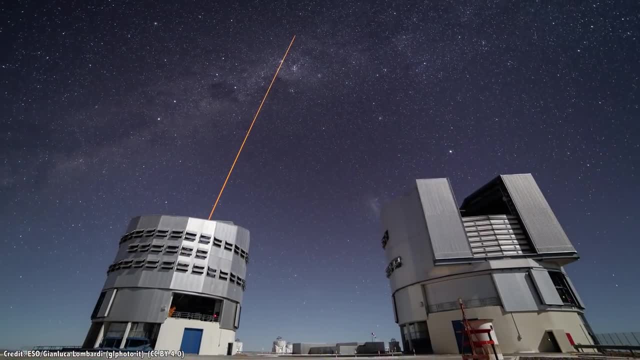 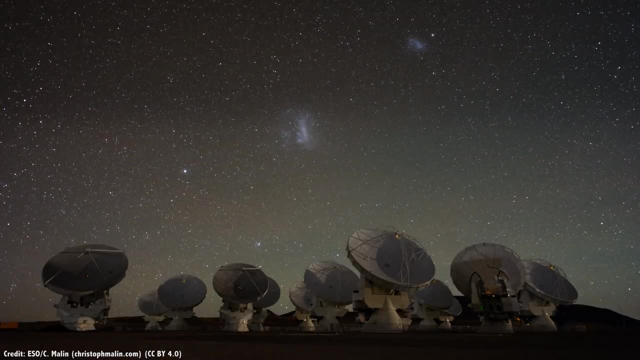 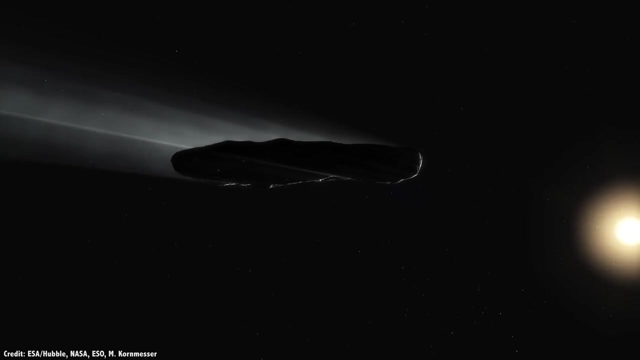 But then maybe it still means that only Earth ever evolved multicellular organisms. Single-cellular life might be everywhere, but only Earth has animals and intelligence. Of course, so much of this is going to remain purely theoretical for a very long time. Even if we could sample interstellar comets, a tiny fraction of them would contain any. 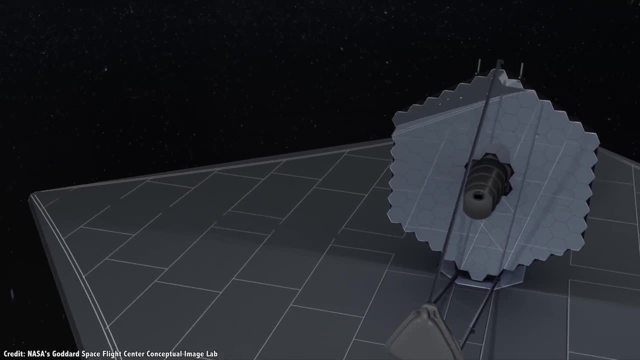 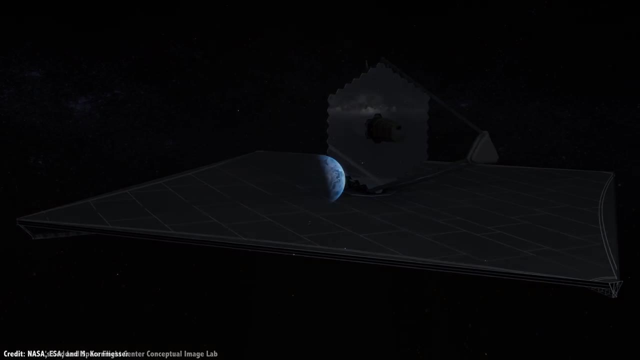 interstellar bacteria. And if we do perceive faint biosignatures in the next generation of monster telescopes, we can't actually perceive their DNA yet. The only way to know once and for all is to send a mission to another star and actually 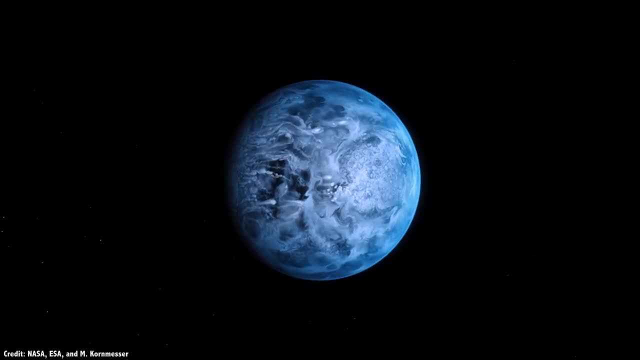 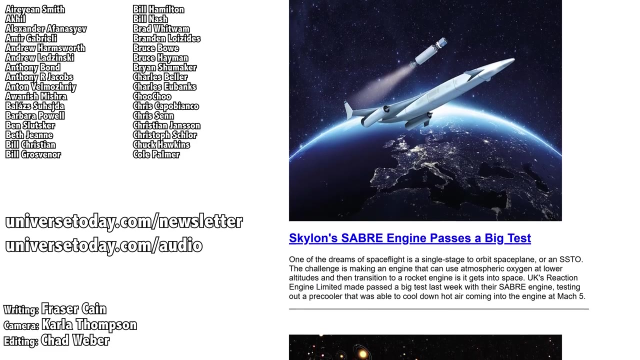 sample them directly And, of course, if we do, we'll send our bacteria with us. What do you think? Let me know your thoughts in the comments. Here are the names of the patrons who support us at the $10 level and more. 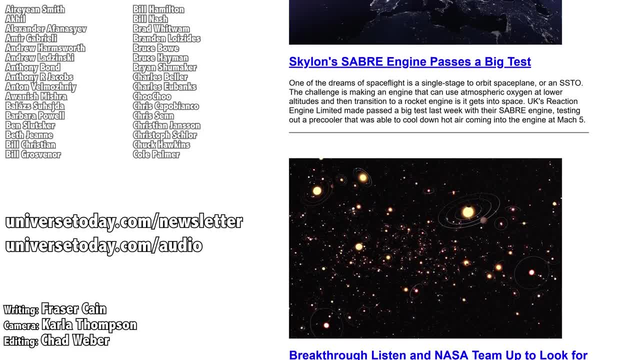 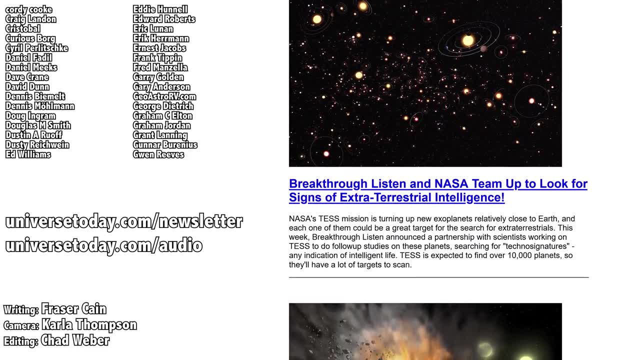 Want to see your name here and support the work we do. Go to patreoncom slash universe today. Once a week I gather up all my space news into a single email newsletter and send it out. It's got pictures, brief highlights about the story and links so you can find out more. 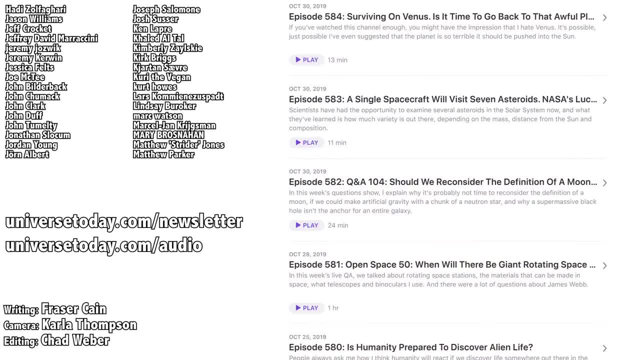 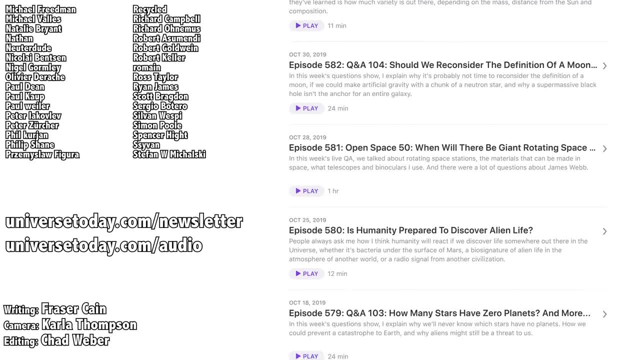 Go to universetodaycom slash newsletter to sign up. And did you know that all of my videos are also available in a handy audio podcast format, So you can have the latest episodes, as well as special bonus material like interviews with me, show up right on your audio device. 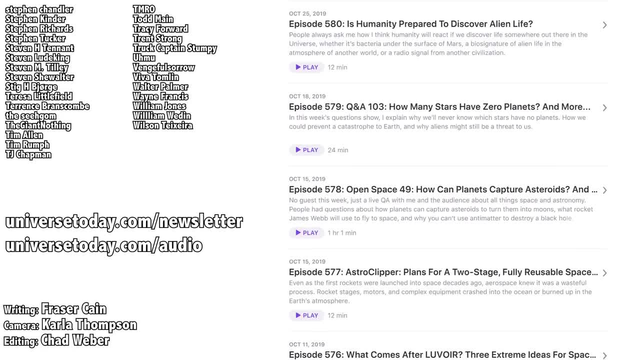 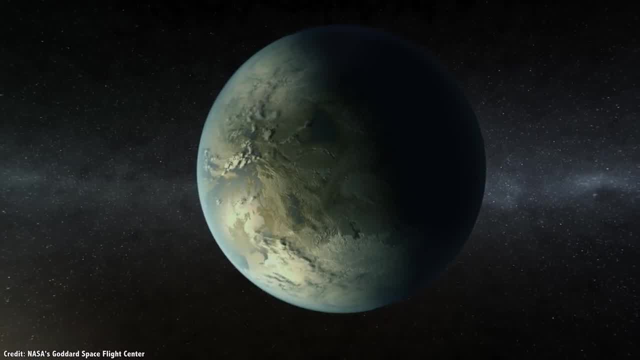 Go to universetodaycom, slash audio or search for Universe Today on iTunes, Spotify or wherever you get your podcasts. I'll put a link in the show notes. Observing another world and even knowing if there's life, there is going to be a difficult.